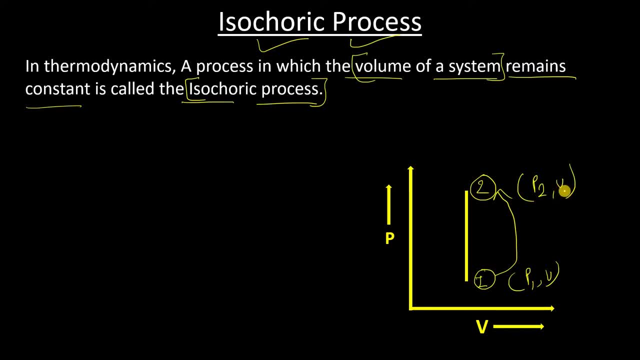 here. we can also say that P2, V, and we can also say that: suppose this is my V2 and this is my V1.. So what I will say? I will say V2, V2.. V2 is equal to V1, at which case this can happen and this PV diagram can become. 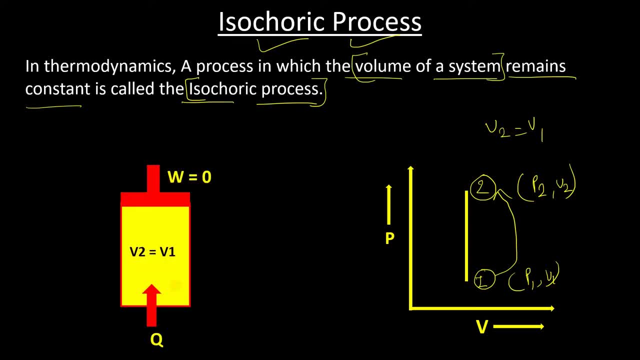 So we can simply say that suppose we have a system, okay, Suppose this vessel we have and this is our rigid vessel. We can say: if we have a rigid vessel or any system that is rigid, okay, At that case. suppose I am supplying here Q amount of heat. 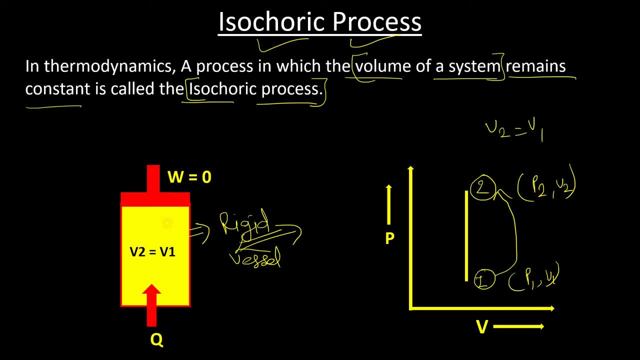 Okay, I am supplying here Q amount of heat and my this system is rigid. okay, So, while supplying the heat, what is happening here? My pressure is going to change. Suppose my pressure is increasing. okay, Because I am supplying the heat and my temperature is also increasing, but my volume is constant. 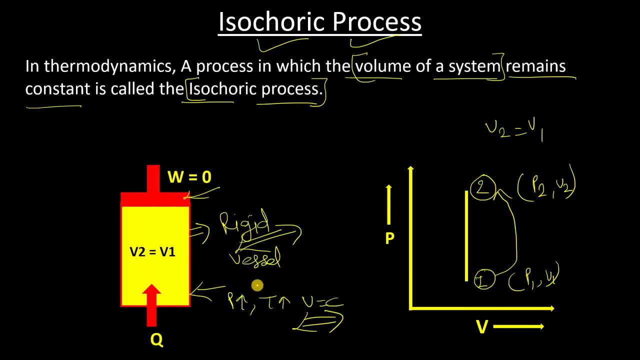 That's why the initial condition and the final condition is same. That's why V2 is equal to V1 is here, right, But pressure and temperature will change. Got it my point? That's why I have written here: W is equal to zero. 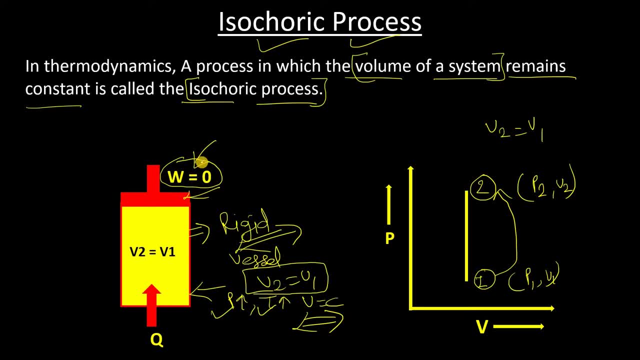 Why? Because we know that for doing some work or to get some work, we will have to expand or compress our system. okay, And we should have some movement, but there is no movement because of the rigid body. So that's why this W means work done. 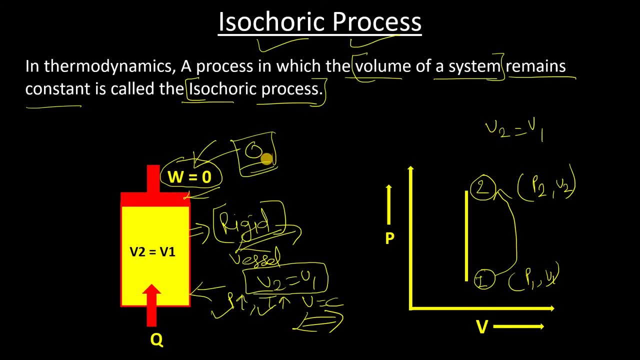 That is why we have to expand and compress our system. okay, So now let's go to the next question. now the question is: what is the ideal gas relation? The ideal gas relation will be 0. In the case of the isochoric process. this is the practical application, okay. 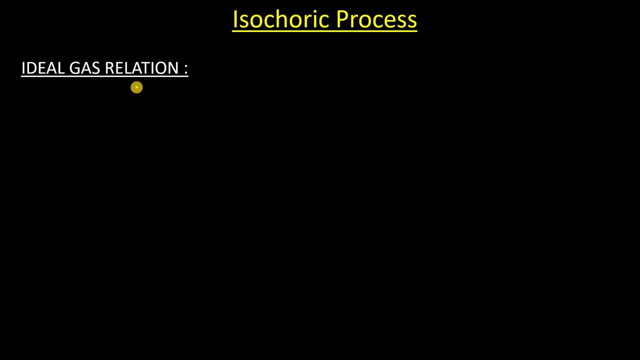 I will also tell you about the theoretical concept as well, for the isochoric process Got it. So this is about the isochoric process. What is the isochoric process Now? see here: PV is equal to nRT, we know that right, and for one mole we can simply write PV. 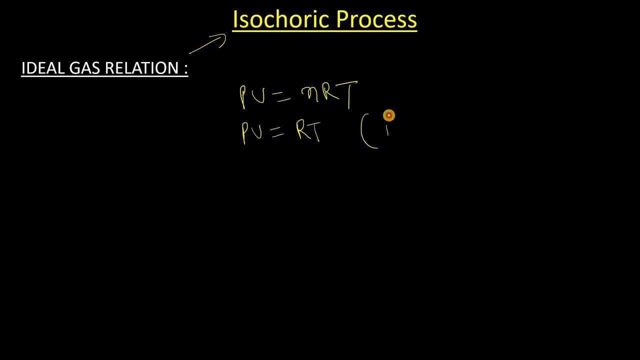 is equal to RT for one mole, right? so here we know that our V is constant and our R is also constant. then what I can write here? I can write here: P by T is equal to R by V is equal to constant. got it my point, what I want to say? okay, if I. 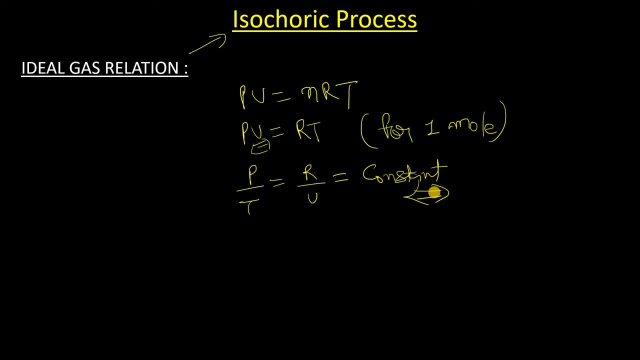 further expand this ideal gas relation in the PV T relation, then what I'll get? I'll get the here. see here, like I know that my P by T R is constant, then what I can write here I can write here: P by T is equal to I. 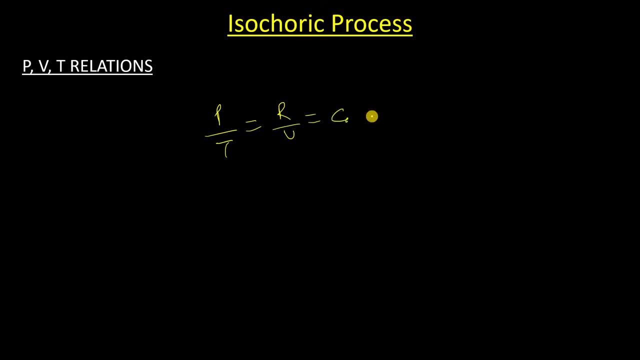 equal to R by V will be constant. okay, the C is a constant. okay. so suppose my system change its position from 1 to 2 means state 1 to state 2. then what I will get? I will get: P 1 by T. 1 is equal to P 2 by T 2 is equal to constant. I. 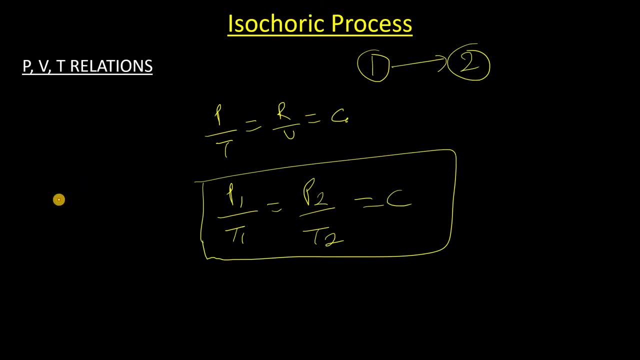 hope you got my point okay. like we know, the one relation, that is, P 1, V 1 by T 1 is equal to P 2, V 2 by T 2. okay, so we know that our volume is constant, so this term will be cancelled out. then. P 1 divided by T 1 is equal to P 2 divided. 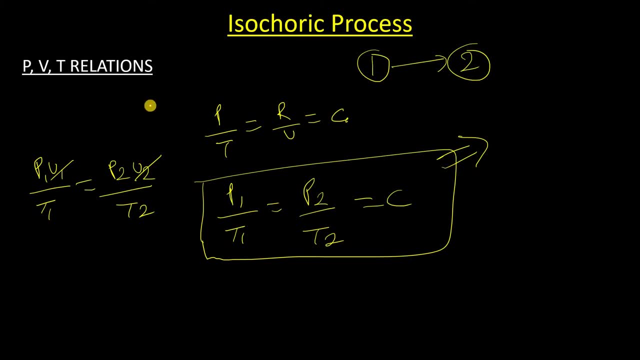 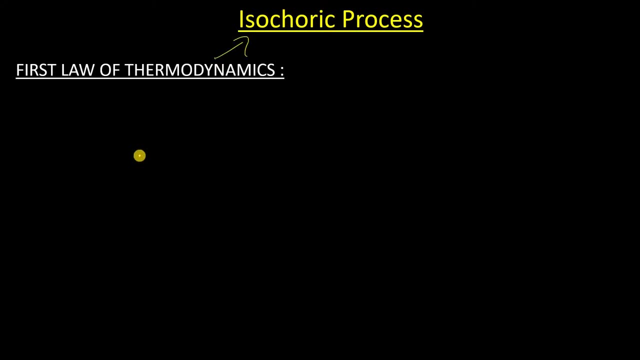 by T 2. so this is our PVT relation for isotropic process. now for the first law of thermodynamics. what is our isotropic process? so for the first law of thermodynamics, we know the like fundamental equation of the first law of thermodynamics, that is d? u is equal to d. 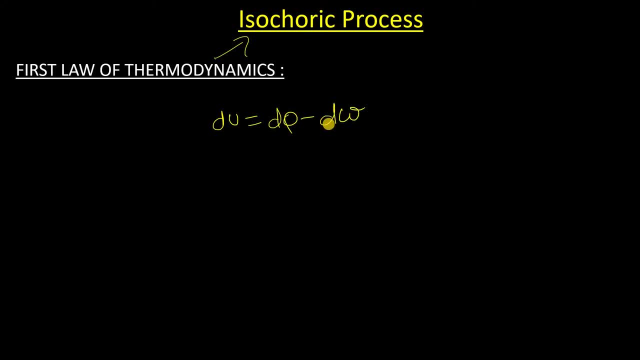 Q minus d W. that is a general equation, got it? so, as I have told you earlier that this d? W will be 0, because our system is neither expanding nor compressing. so that's why what will happen, d? u will be d Q. okay, that is all. 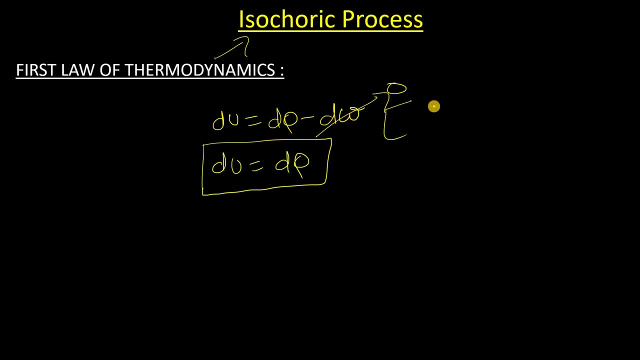 okay. so why this d W will be 0? I am telling you here: we know that our d W, okay, it will be p d v, okay. so this differential is going to be 0. this differential is going to be 0, why? because it's not going to change if this. 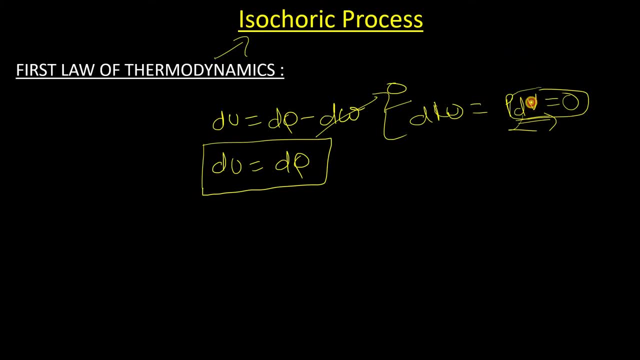 is not going to change. so we know that the differential of any constant value is 0. that's why this d W will be Ô 0. Now here, du is equal to dq. then what will be the value of du? Then I can simply write that du is equal to dq is equal to nCv dt. when I integrate this, 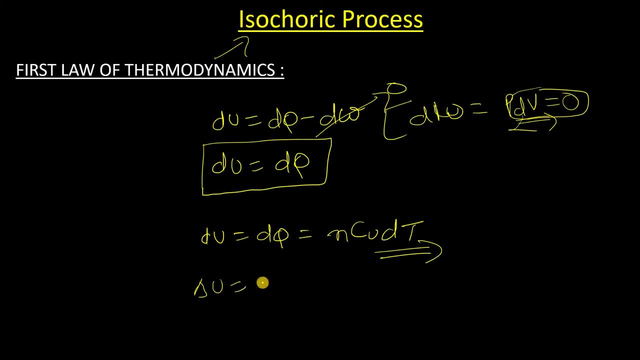 one, So that I will get: delta u is equal to q, nCv, delta t, and this delta t can be written as t2 minus t1,. got it Because this is the change in temperature and same here that is change in internal energy. 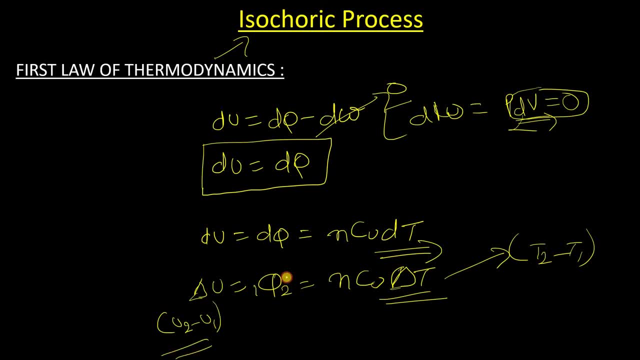 it will be also u2 minus u1, I can write it, But I cannot write my heat as delta q. why, If you know that? why, please let me in the comments box If you do not know why. so I have uploaded one video on path function and state function. 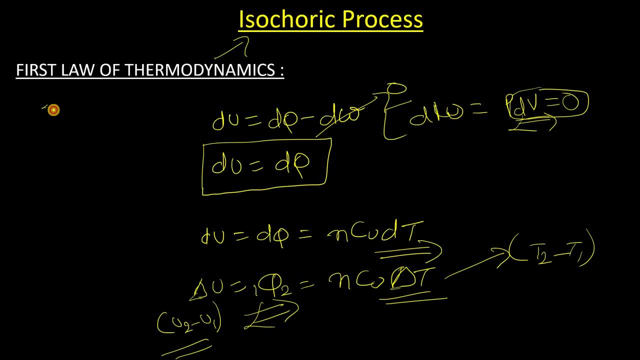 Please watch that video and you can also watch the videos on first law of thermodynamics. Okay, so I hope you understood that. what is the isochoric process for first law of thermodynamics? It is very, very simple. okay, If you know this, then you can write it. 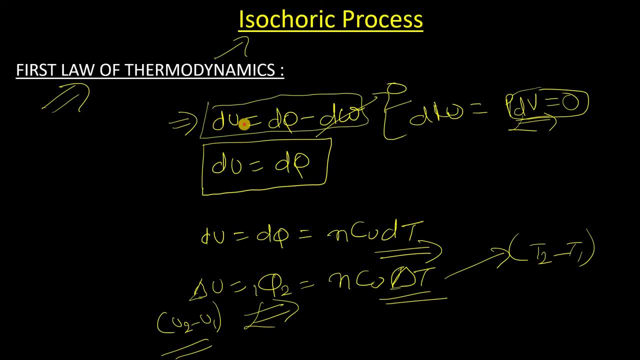 If you know this fundamental equation, then you can solve it very easily. But if you do not know, then you will not able to solve. got it. And if you know the formula for the du, du means this formula, if you know, for the internal. 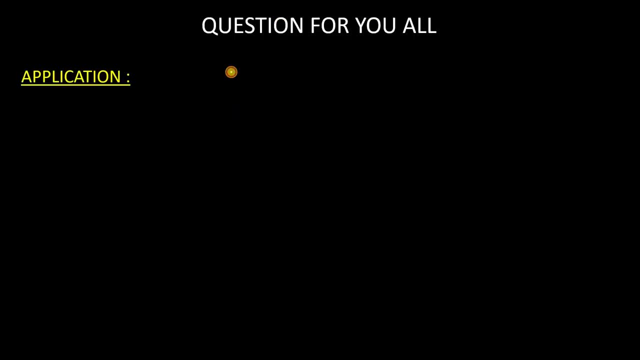 energy got it. Now here is a question for you all, and the question is that what is the application of the isochoric process? There is a one application for the Otto cycle, But let me in the comments box The more example and the more application of the isochoric process. So thank you for watching the video. See you soon.